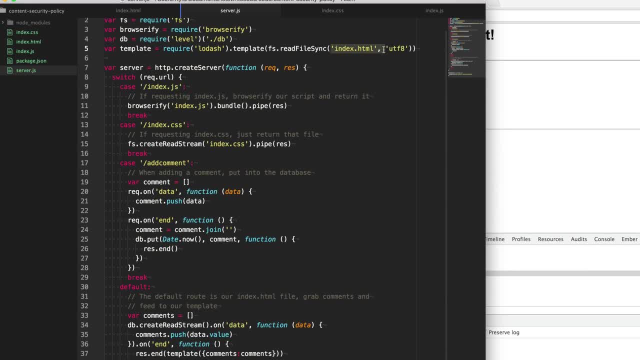 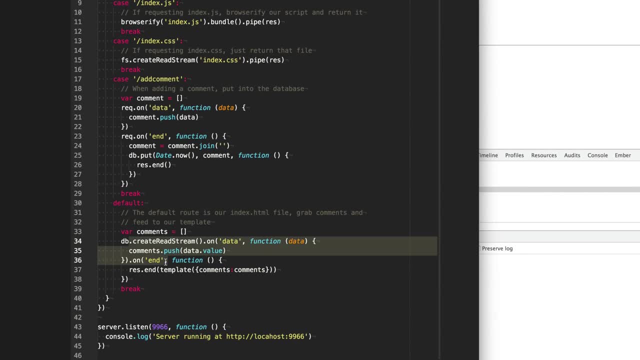 we're just going to serve off our template here, which is our index file. that gets rendered using this Lodash template here And it feeds in all the comments that we get from the database here, And how this is all constructed is really, again, not important. It's just an example app. 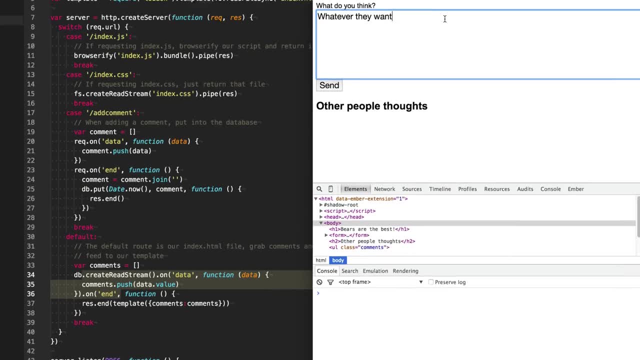 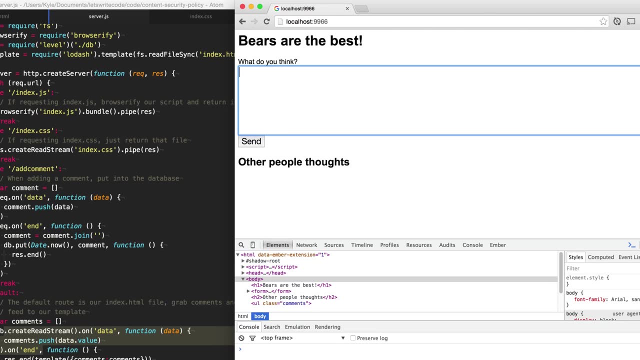 just to show you some of the security concerns around it. OK, so we have this simple form in which we want users to input what they think about bears, And this might be hard to believe, but some people on the internet are not very nice And they may. 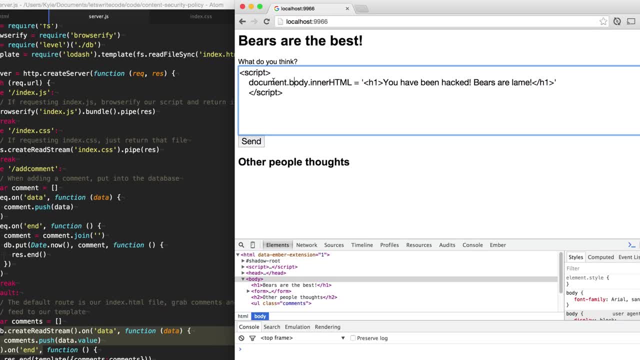 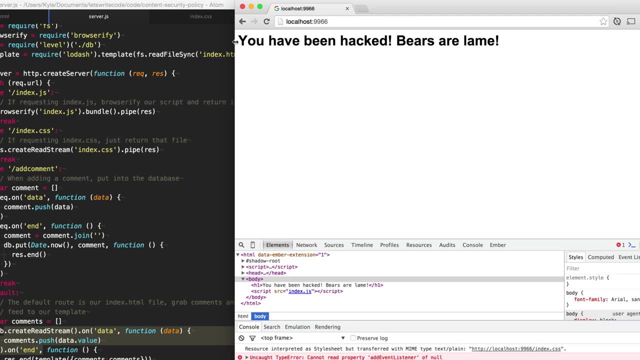 enter something of this sort a script tag with the document body, inner HTML set to their own message, And so when we send this through, you'll see that our website has been hacked, And even when we refresh, this is the message we get. 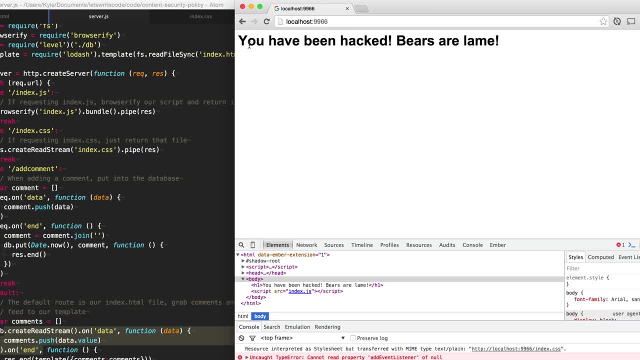 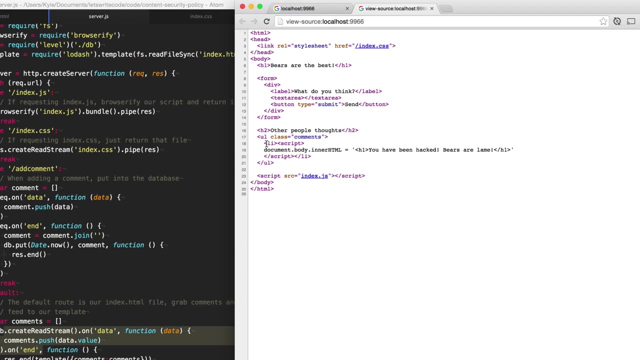 Any visitor that goes to our website will get the same message too. That's not right. I don't want people to think that bears are lame. I don't think bears are lame. So if you look at the actual source of the website, you'll notice that it is our normal source code, except that in here, where 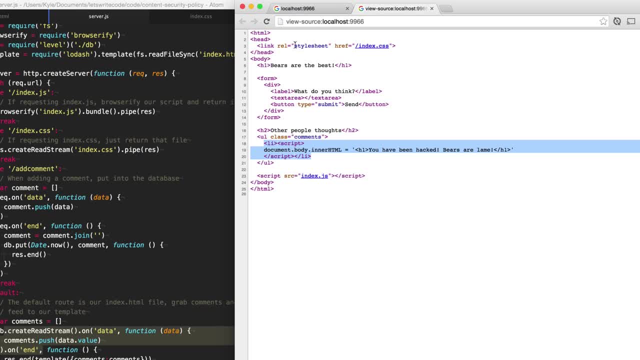 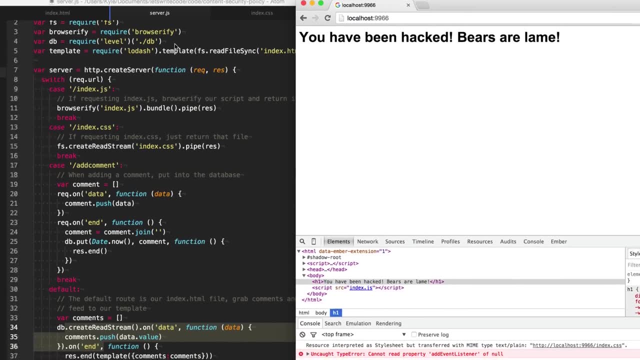 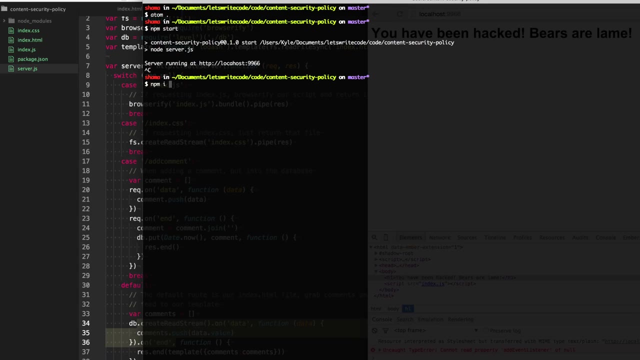 it's supposed to display the user's comment, it's injecting this script tag. This is known as a cross-site scripting attack or an XSS attack. So one way to fix this is to sanitize the input as it comes in before it reaches our database. So there's many sanitization libraries. 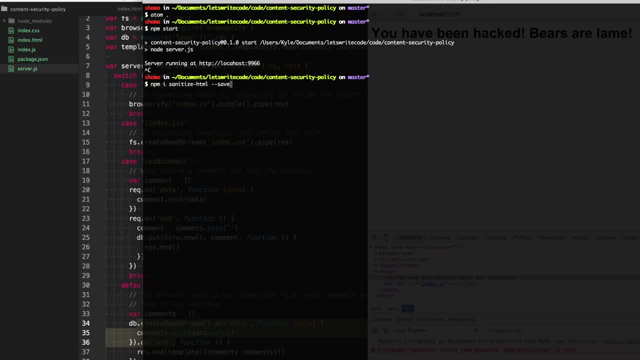 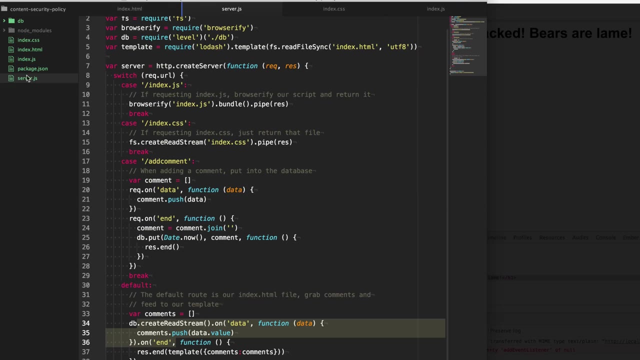 on npm. I'm going to be using this one called sanitize HTML here And I'm going to type npm i or npm install, sanitize HTML to install it And start my server back up here again. And then I'm going to go here to our server And before it inputs our comment here into the database, I'm 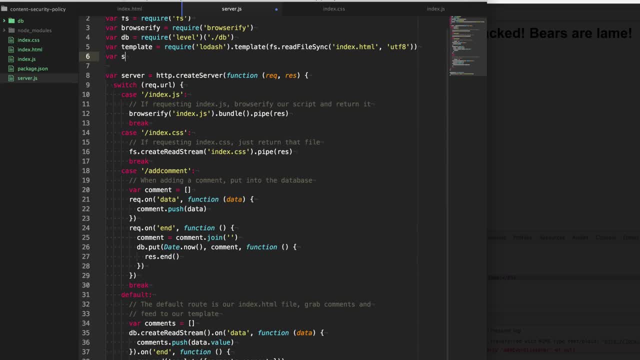 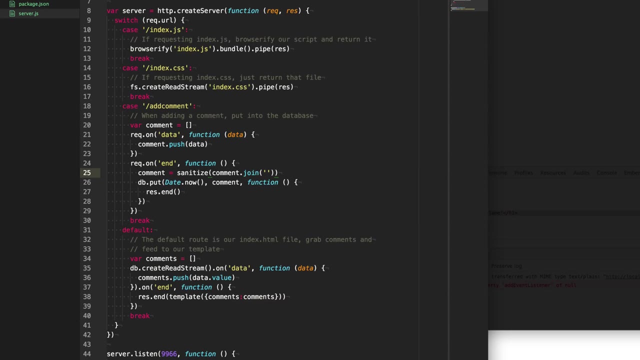 going to sanitize it using this library, So we'll require it up here: Sanitize, Require, Sanitize HTML, And what this will do is it'll strip out all of those nasty HTML stuff that we don't want. We just want normal text contents. And so then now, when we go back and refresh our server here, 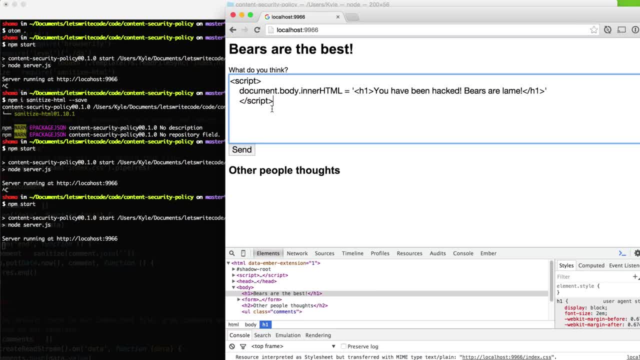 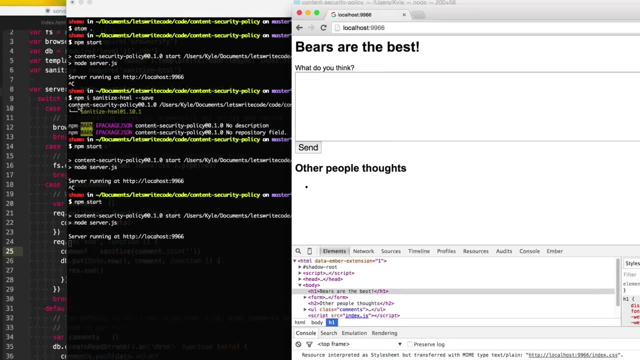 and then go back to the site and insert into this attack here you'll see that we no longer get it. Before it enters our database, it strips out that script tag. So that's one way to do it. Another way to do it that we could do is: 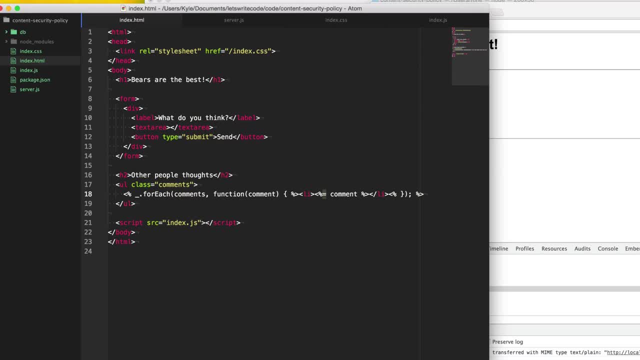 Lodash by default, or when you use this equal sign here, it inserts the HTML unexcaped, But instead, if you use this, you can escape the HTML. So there's one way to do it when the user's input's coming into the server And there's another way when it's coming out. 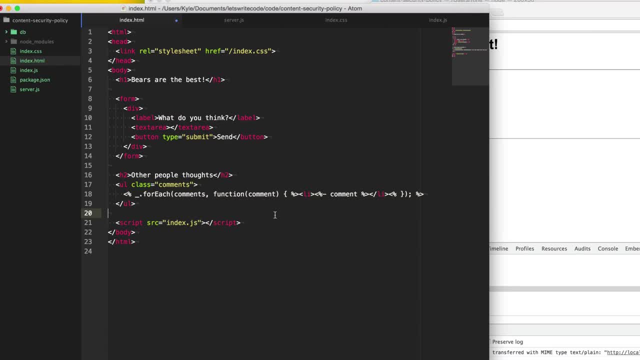 And each of your- depending on your template library and whatever you're using- will have different ways of escaping any kind of thing that's displayed, And really you should be doing both: You should be escaping when it's going in and sanitizing when it's going in, and 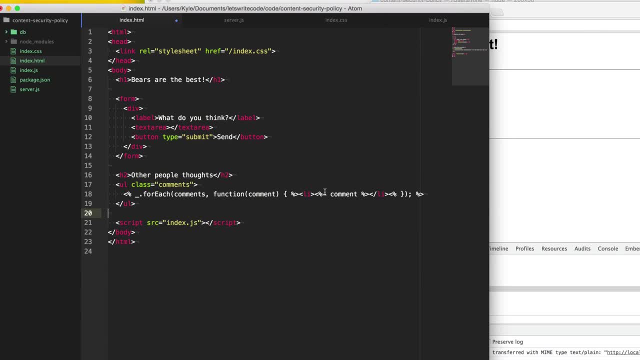 escaping when it's coming out. Just in case somebody managed to inject something in your database through some method, it still won't be displayed on the output, and the vice versa. Now, this app is very similar. It's simple, It doesn't really do much, And most apps are not that simple. They do a lot of things. 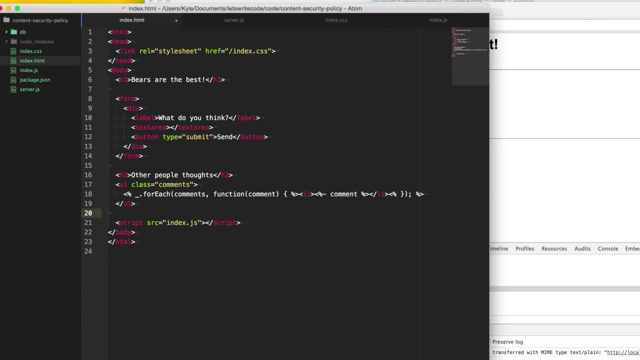 And so 99% of the time, you really don't want users to run their own script tags on your site. So wouldn't it just be easier just to disable all of that in the browser? And that's exactly what a content security policy does. So I'm going to remove the escaping here. 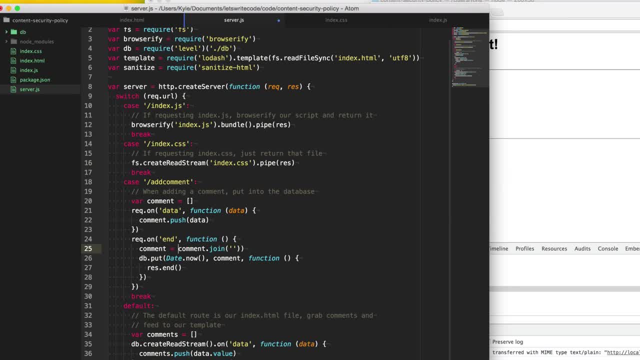 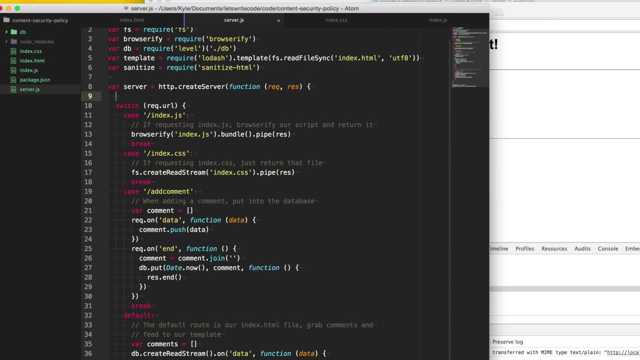 And remove the sanitization here server. all we need to do is we need to send an HTTP header to the browser to tell it to enable this content security policy, And so it doesn't matter whether you're using Ruby or Python or PHP or any server. really, each server has their own method of responding. 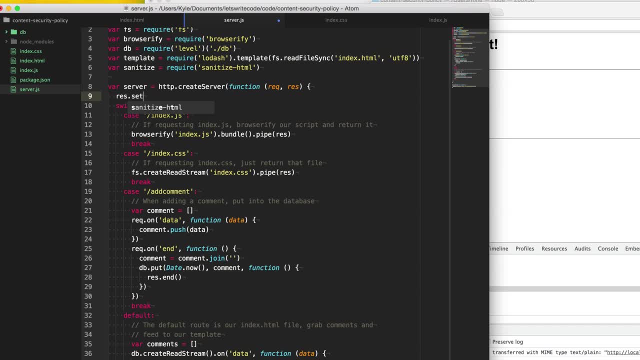 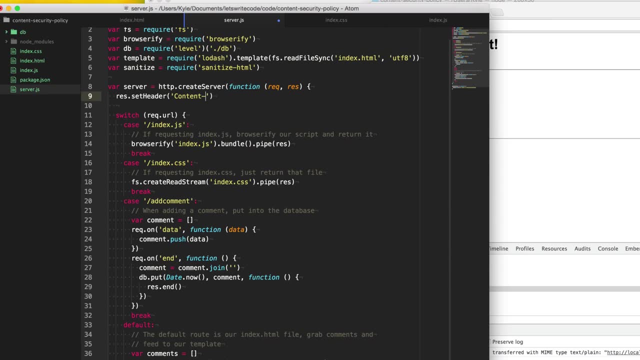 with headers Here, with Nodejs, we can do the response. we can say: set header here and we can set the response header here. And so one of the headers I'm going to set is called content security policy, with dashes in between. And then what I'm going to do. 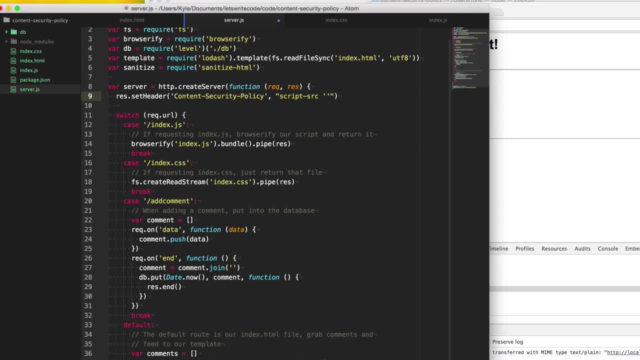 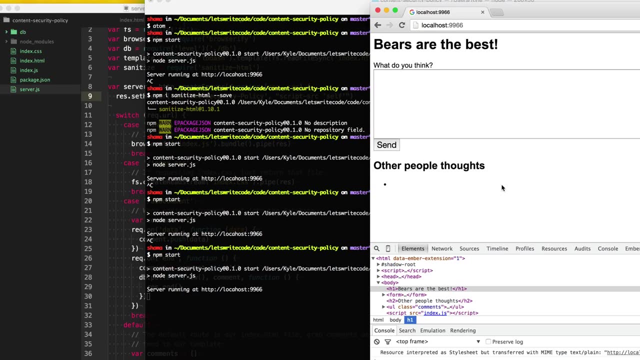 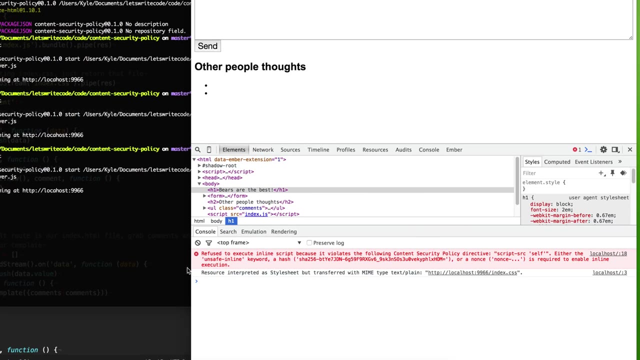 is. I'm going to set a script, dash source and in quotes to self. Now I'm going to go here to my server and I'm going to restart it And then go here to my website, refresh the page and try this attack once again And you'll see here at the bottom, here our browser has. 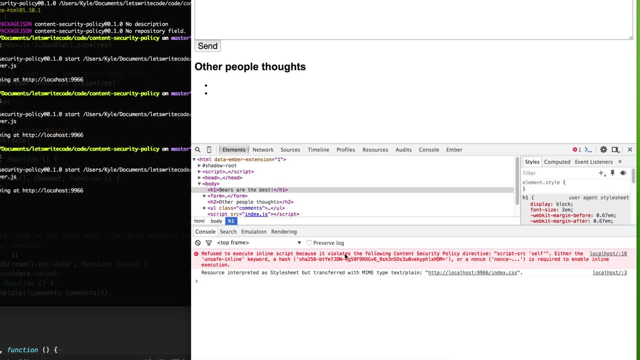 refused to execute the inline script because it violates the content security policy, And so we don't have any sanitization going on right now. but it's recommended that you do sanitize. you still continue to, But in case maybe we missed a part that we didn't. 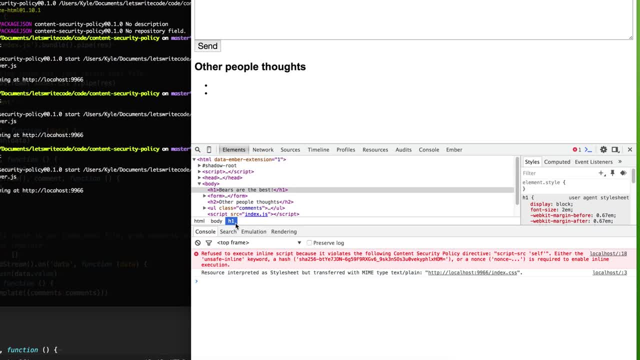 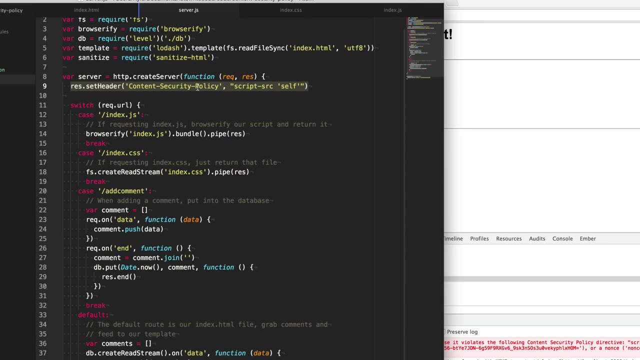 sanitize, or the attacker has figured out a way around our sanitization. the browser still here didn't allow this attack to take place. So just with one line here, one line we're adding here, we have mitigated so many different attacks And so we're going to go ahead and 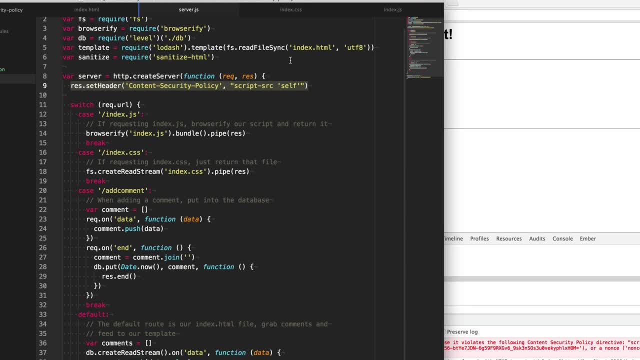 see what attacks that could have been done on our browser. So currently our policy disallows any kind of inline scripts or script sources that don't come from self or it's our own domain. Now there might be instances where you actually want scripts to be injected or come from other sources, such as if you're using Google fonts. 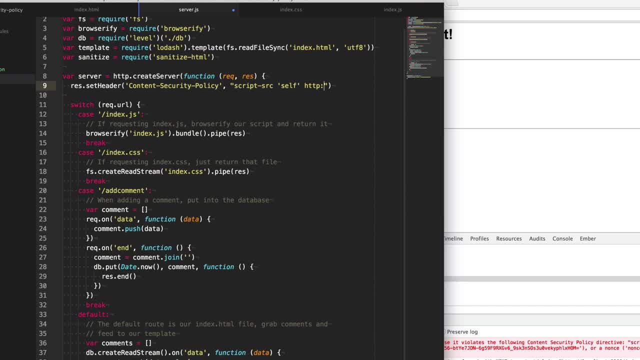 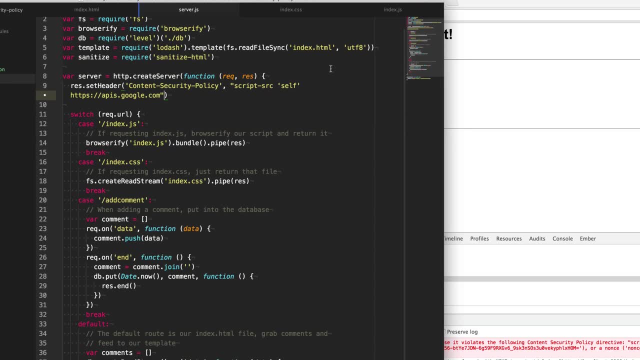 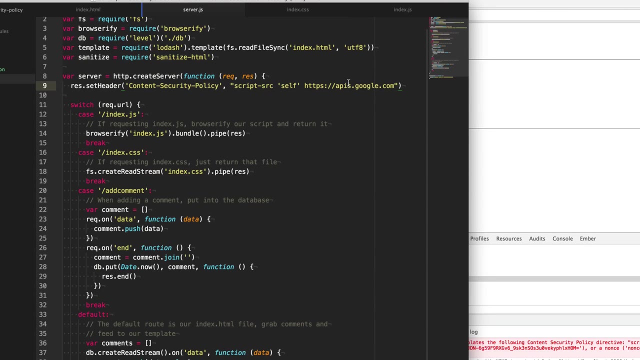 Then what you would simply do is using a space to separate it. You specified the domain name that you trust, So we can say APIs, googlecom here and we can add that to our content security policy. And so now, if Google needs to add any scripts in order to run, it will be allowed. 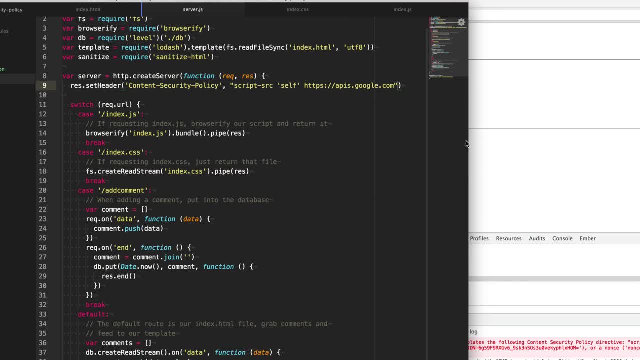 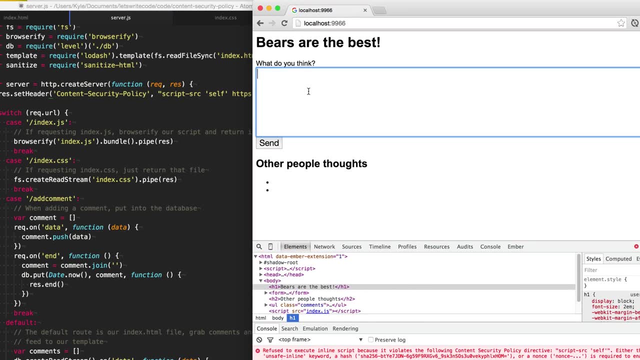 to do so. So that takes care of JavaScript. but now what about CSS? Many people look over style sheets as a potential security threat, but let's go ahead and check our app here, And I'm going to insert in something else that's a little bit more malicious. here Bears are. 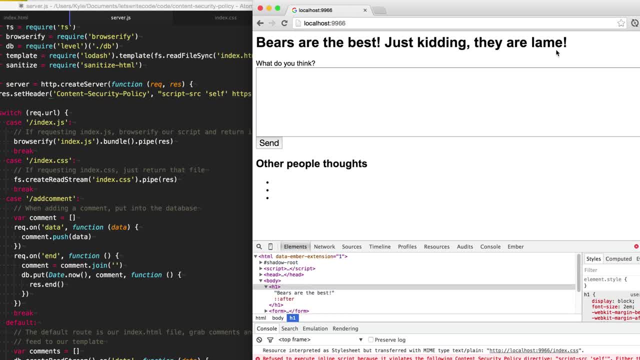 the best. Just kidding, they are lame. Oh no, Using a CSS attack here, they have hacked our website once again, And anybody that goes to it is going to think that I'm just kidding, that they are lame, and that's not what I think. So we need to make sure that this doesn't. 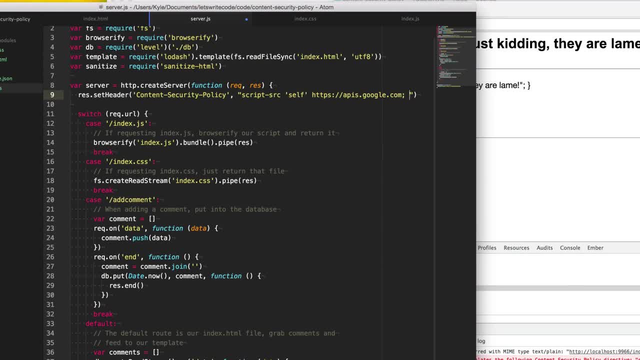 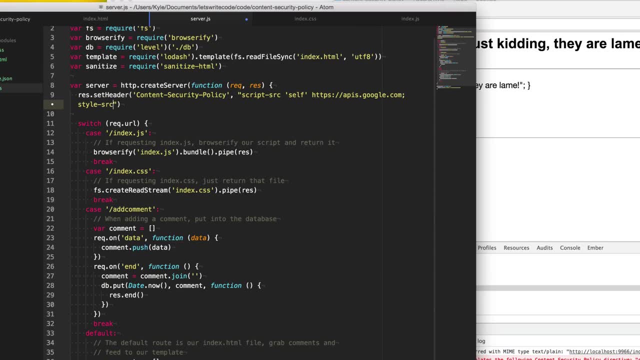 happen as well, And so we do the same thing, but instead we're going to put a little semicolon here to say that we're going to specify a new rule here And we're going to say: style-source is self, And so that means we only want styles to come from ourself as well and not allow any of 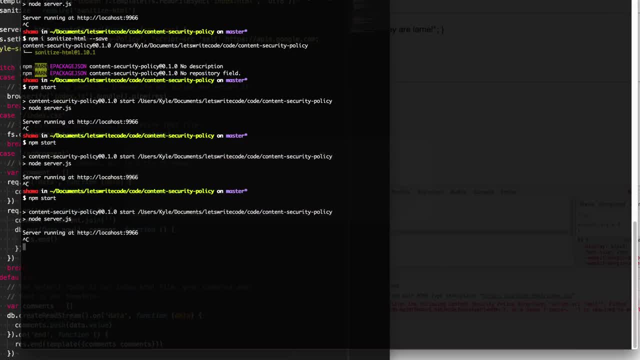 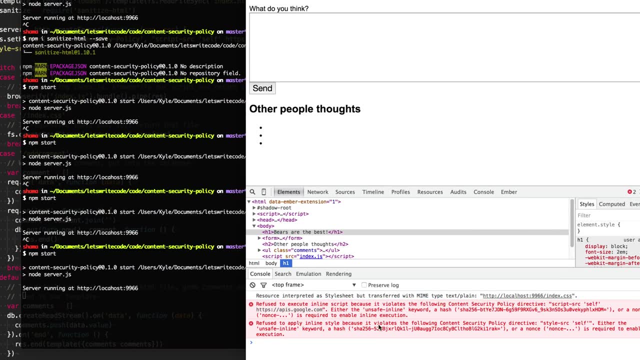 this inline stuff going on, And so now, when we go here and roll our server and refresh the page, you see that it also has refused to apply this inline style because it violates our content security policy- Exactly what we want. They can't hack our website using style tags either. 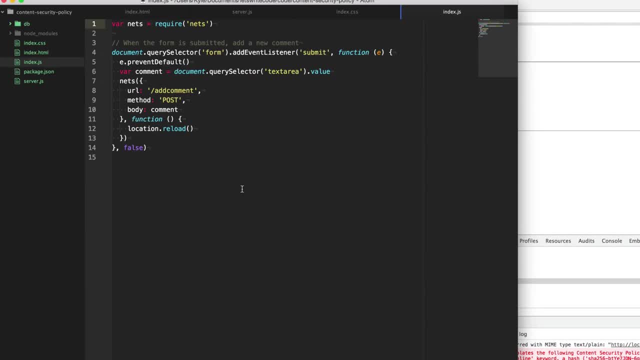 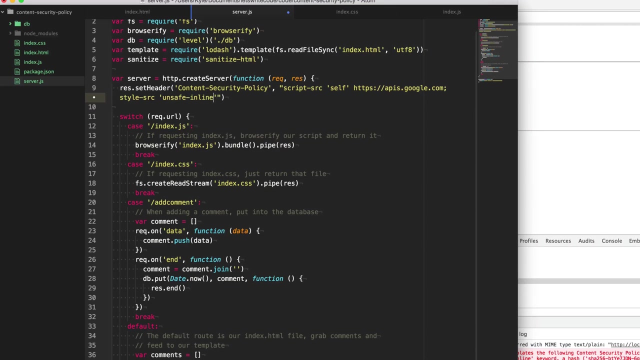 So now this does block inline styles on our page, And inline styles have become a very a lot more popular. They're more frequently used now, And so there might be some instances where we don't really want to block them. Now we can. there's settings in our content security policy where we can say: unsafe inline. 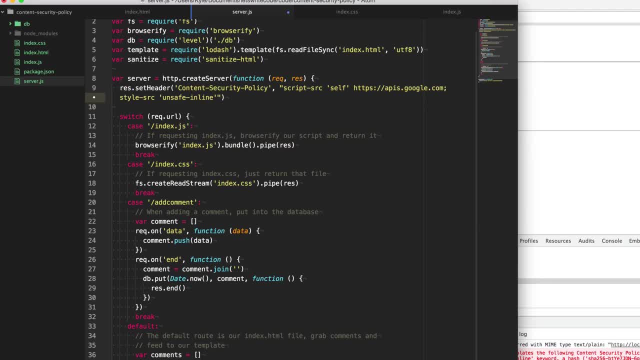 That basically allows us to put unsafe inline styles, And we don't want to do that, though We want to. just we want to work around our own kind of thing here. So let me give you an example of what an inline style would be. So we have this H1 tag here, for bears are 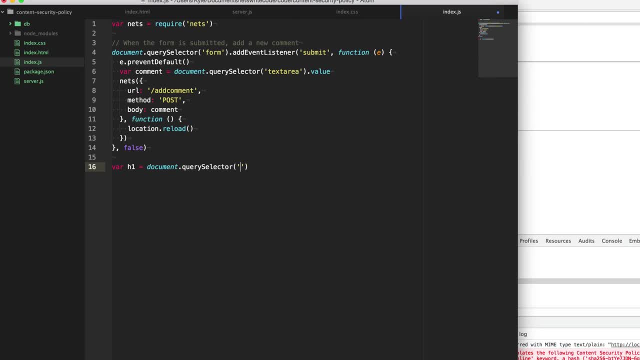 the best here And I'm just going to query selector it H1 here And then maybe you know I'm doing, maybe I need to do some kind of calculation- that can only be done once the JavaScript has been loaded and everything, And we need to detect, maybe like the width. 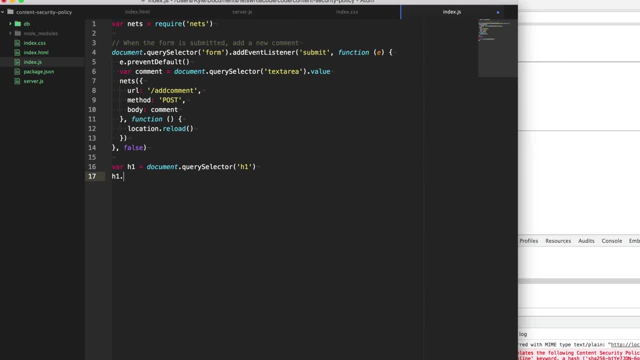 or something to center it, or there's whatever reason. we're setting this, this style attribute, here on on this tag. Uh, we're setting it dynamically and we need to here. So for just this example here, I'm going to set it to red, Um, and then let's add: like a tech shadow, cause it's going to. 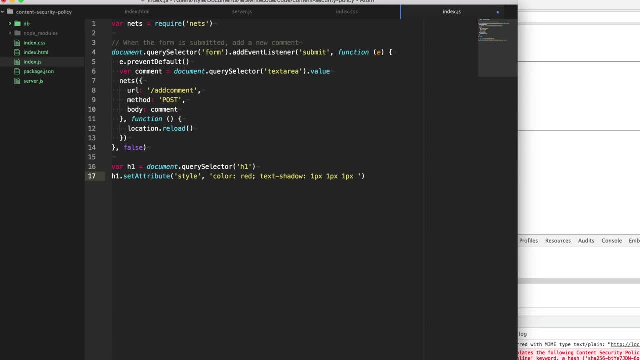 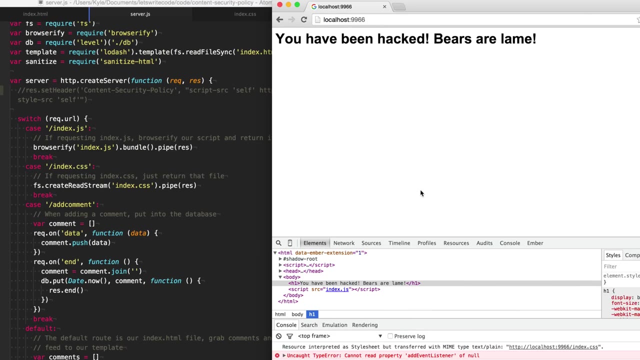 look super, super cool. Uh, I don't know, black tech shadow here. So we're going to set this, uh, this style attribute here And just to show here. I'm going to disable our content security policy and roll our server, just to show what I want it to look like. 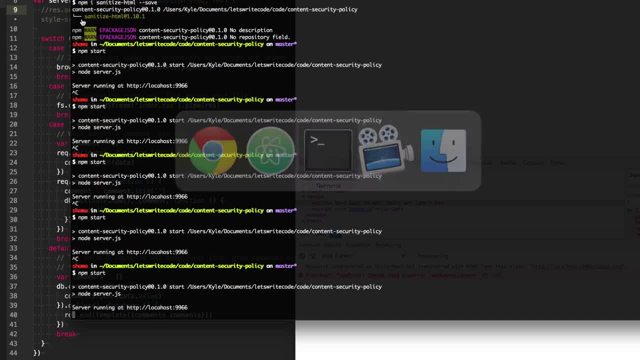 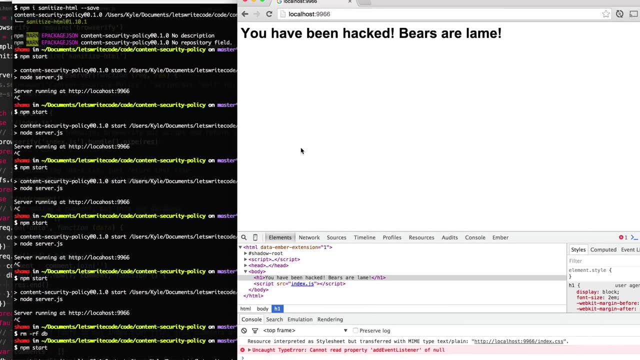 Oh no, we've been hacked, So let me go ahead and, uh, clear this uh database here. first, clear out any, any of that malicious stuff that we've, uh we've been attacked with before. Okay, So now this. 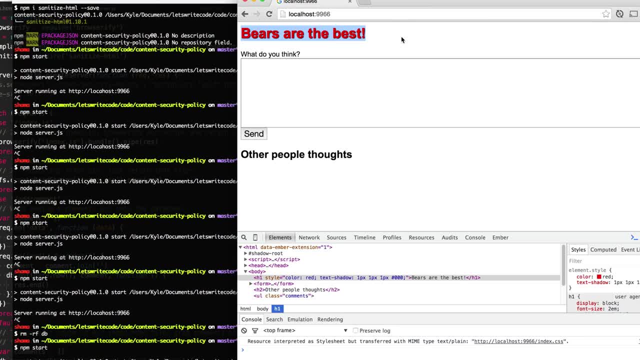 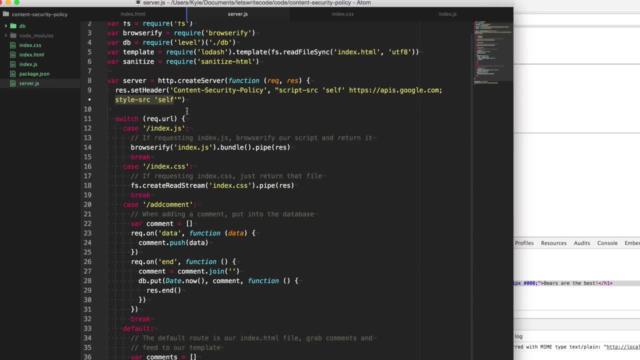 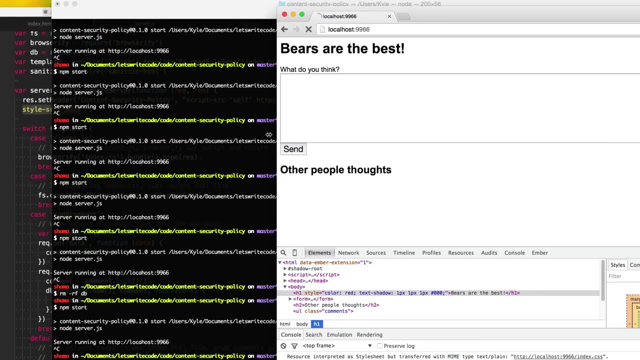 is. this is what we want. uh, cause, that looks awesome. You know it's, it's that. but so now we're going to go ahead and re-enable our content security policy, which includes the style source: uh, self, self, uh, um declaration here and roll our server to get that, And 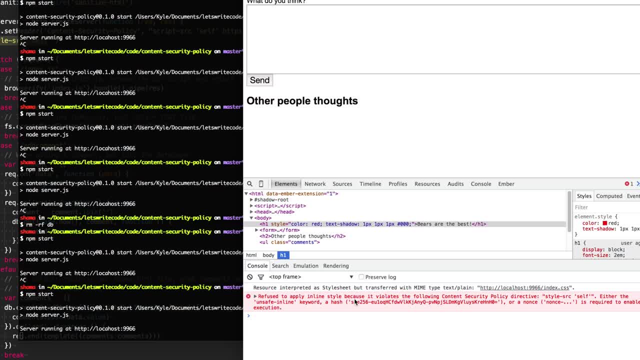 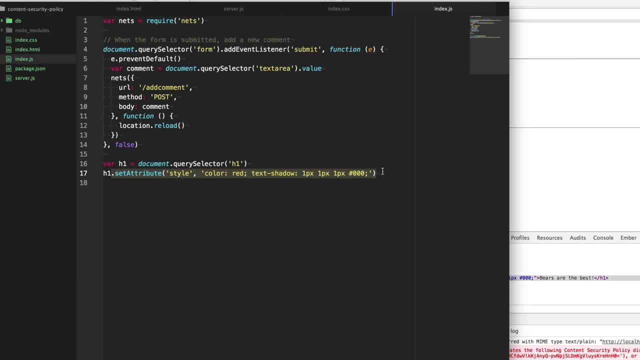 so now, when we do this, Uh, it's refusing to apply this inline style uh to it, because, uh, this part here, when we're setting the style attribute, this is an inline style. This violates our content security policy And it's really simple to get around. Instead of setting the style attribute, 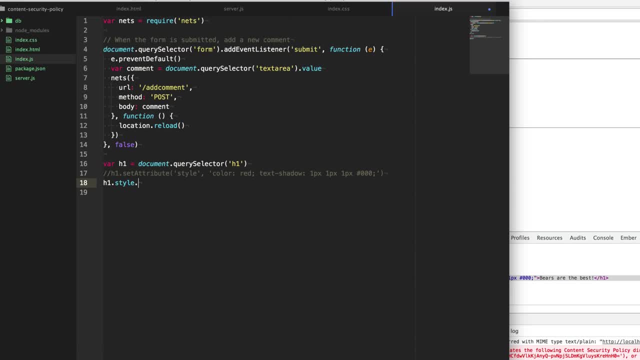 you should set it, uh, directly. um, how you should? So we'll say: style, uh, color equals red H. one style text shadow equals one pixel. Uh, and then we're going to go ahead and do that: Uh, pixel, one pixel, one pixel black. So we're setting this, these, these properties directly. 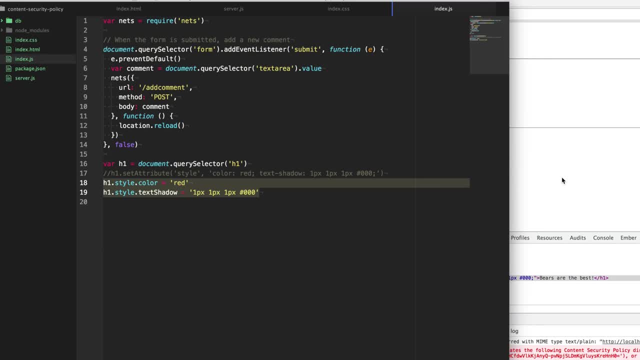 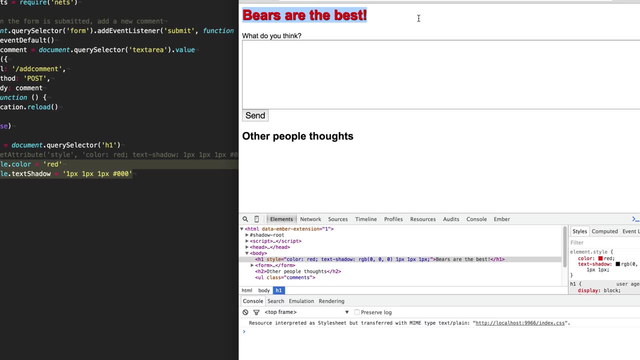 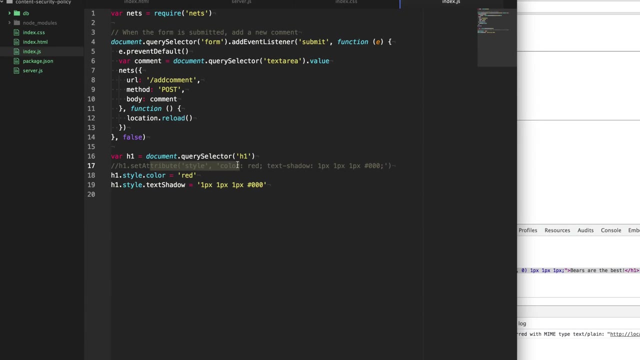 on the style: um, uh, um, object here, And so now, uh, when we refresh the page, you see, even though we have our content security policy in place, we still get the inline styles we want. So it's just slight difference. here is, instead of applying it to the style tag. 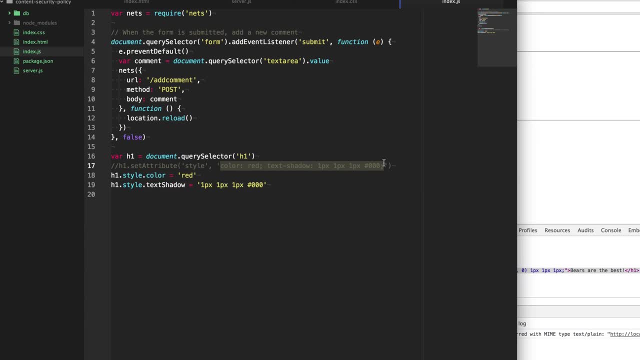 uh, which you know users may. uh, our attackers may be able to inject some malicious code into here. We can simply apply it directly to each of the properties in which uh is a bit more safe. Now, if you, if you're not a really a fan of I mean, maybe you have a whole bunch. 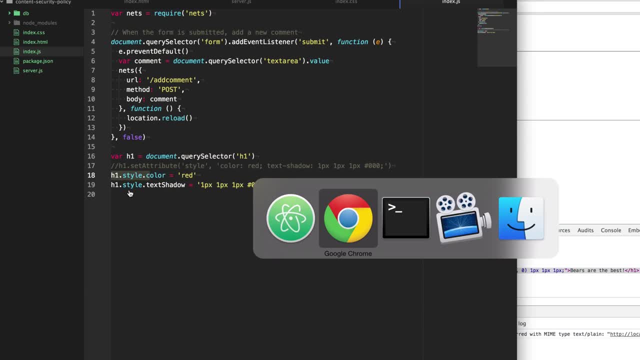 of styles to apply and you're not really a fan of this. Uh, there's a? uh, I got, uh, a fancy trick from um Matt. uh, that's a low year, I don't know how to say his last. 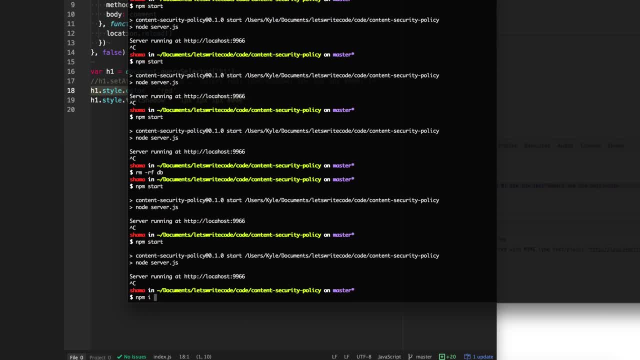 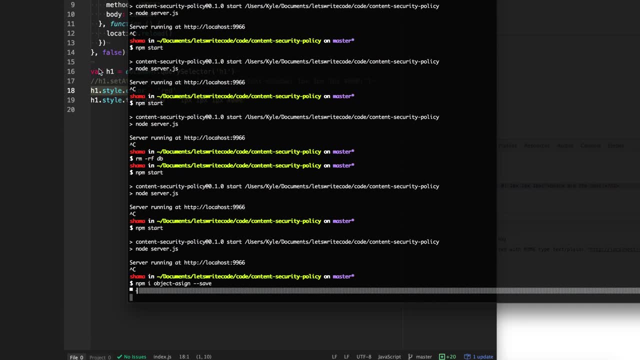 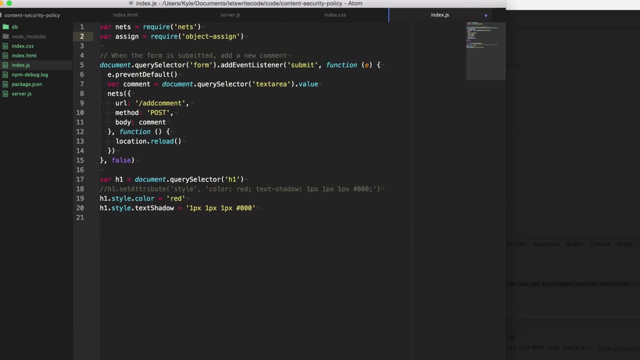 name and I apologize. Um, so what we're gonna do is we're gonna install, uh, we're gonna do NPM, install object assign here and save that to our dev dependencies, and then i'm just going to go ahead and require it here, so we'll say object assign. now, object assign is uh an api that's coming, uh, in newer. 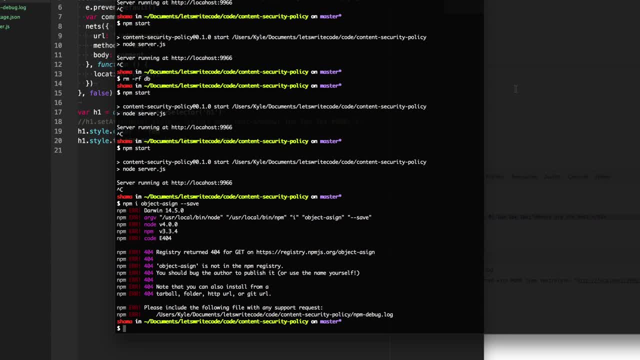 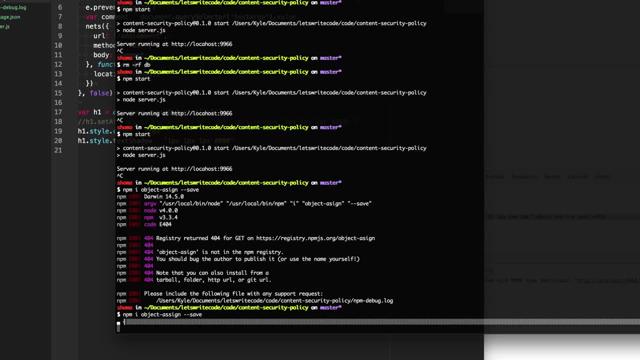 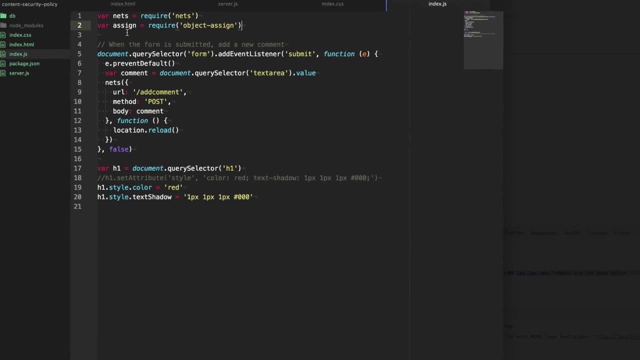 browsers and it may not be available. it's not. it's not available everywhere yet. um, oh, i forgot an s here. uh, let's uh, make sure we spell things correctly with two s's. uh, and i got two s's here, okay, yeah, there's definitely two s's there. let's start up our server here. so object assign is: yeah. 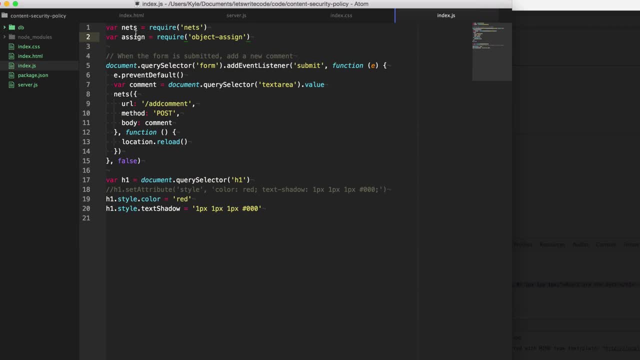 it's a new, it's a new api in in newer browsers. it may not be available here, but uh, cinder source has got us uh covered here with this library that that gives it. you know this, uh, this, this thing that we want here. so, instead of doing it this ugly way, we can do it this way. we can say: assign. 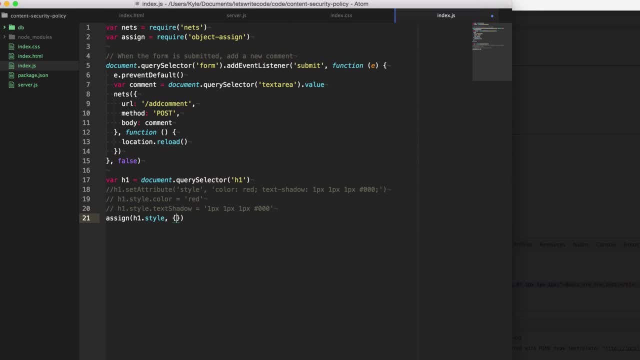 and we're going to supply an object here and we're just going to give it properties that it's going to assign to this, uh, this style object here, so we can say color red and text shadow, and i'm not going to type that again because typing that three times is just ridiculous- and so let's save that and our 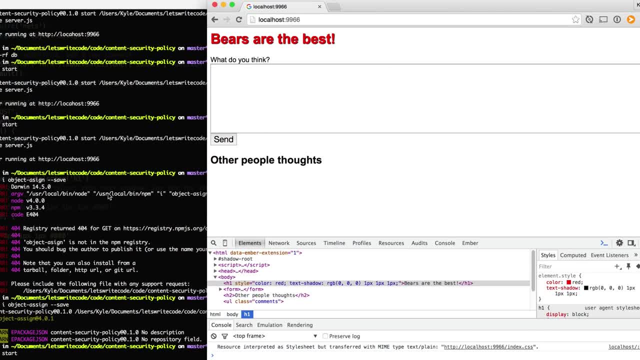 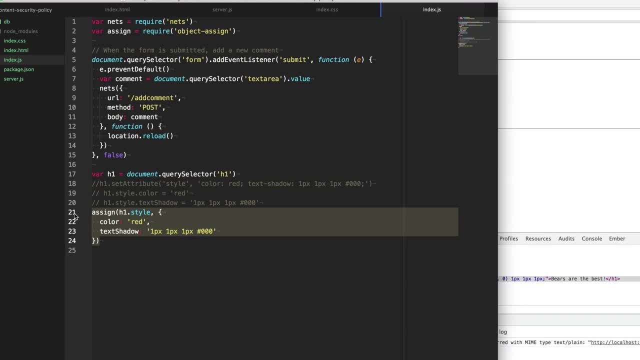 server is running, so let's go ahead and refresh the page, and so this is just a a nice fancier way, and it's still secure and we can set all the css properties in line as much as we want. so i hope this has convinced you to. 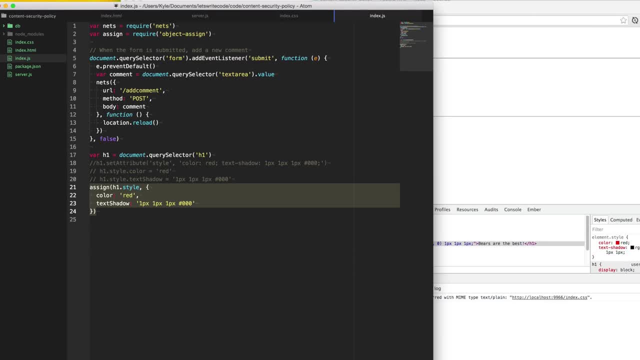 enable the content security policy on your website, and not only should you be sanitizing the input as it's coming into your database or server or wherever it lives, and then escaping the output as it goes out to the browser, but i i really heavily encourage you to enable a content security. 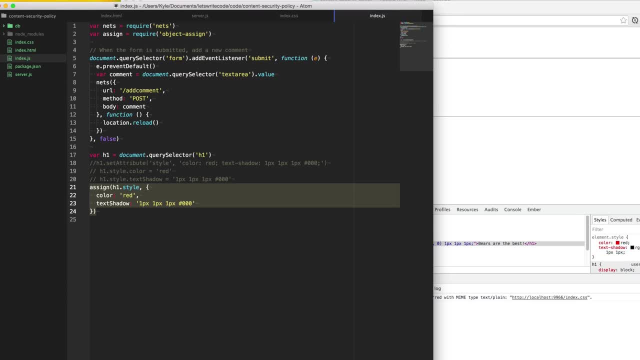 policy for both javascript and style sheets. uh, and just make everything uh make, make your life easier, make everything more secure and don't have to deal with those nasty uh cross-site scripting attacks. um, and if this has helped you, then please share the video and have a great day, and i'll see you in the next video. 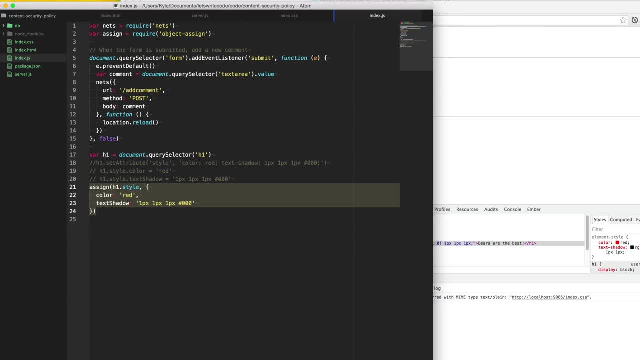 help others and if you want to see more videos, please subscribe. thanks again for watching.